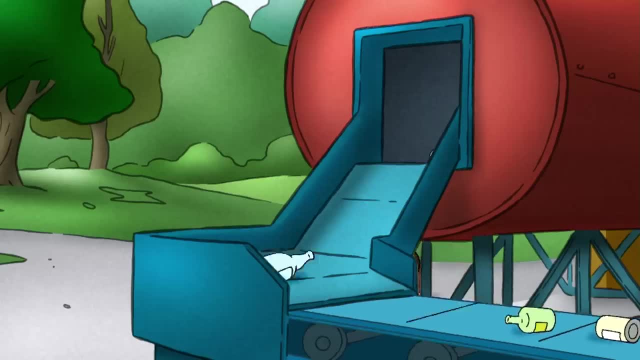 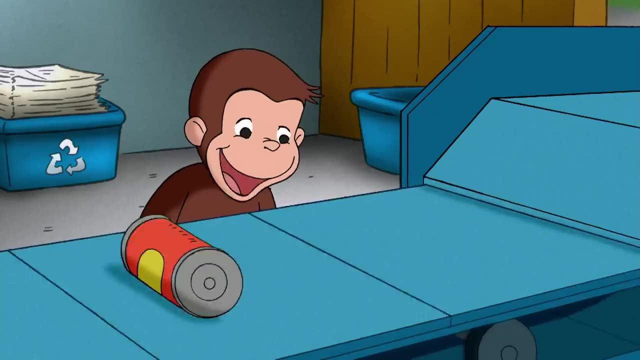 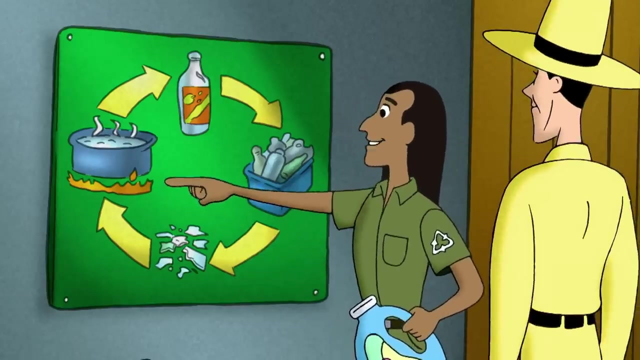 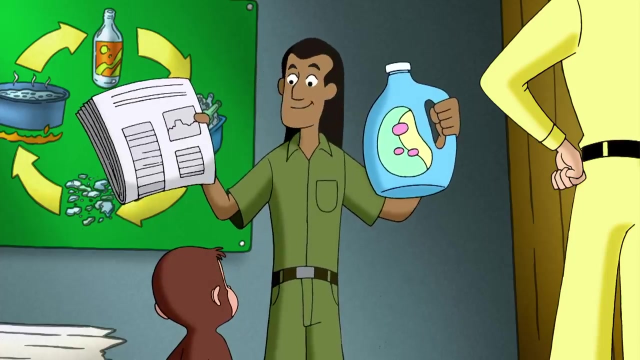 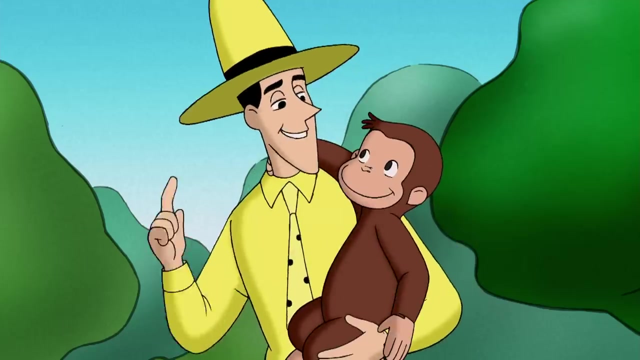 First containers need to be separated, then cleaned. Glass is broken into bits, then melted down to make new containers. Plastic works the same way. Recycled newspaper makes new newsprint. Think you're ready to start recycling Now you can help with the contest. 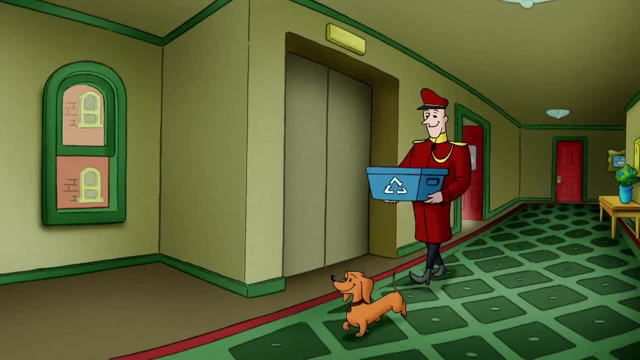 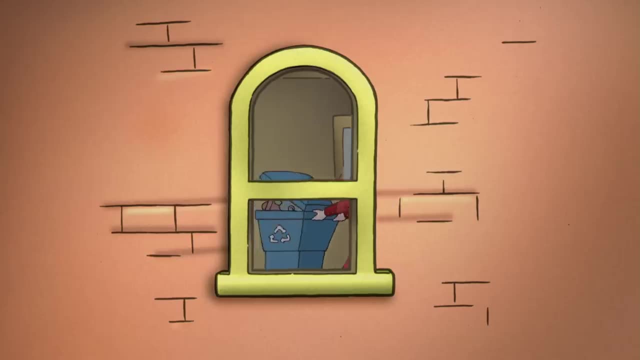 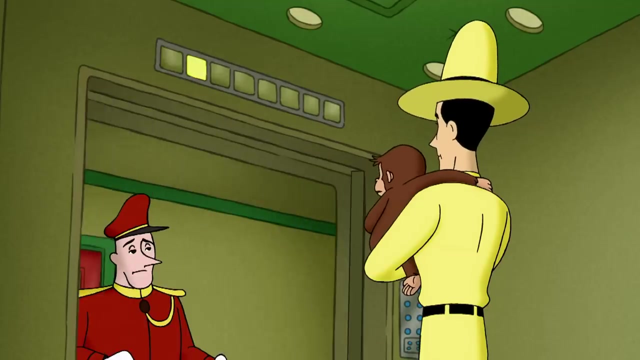 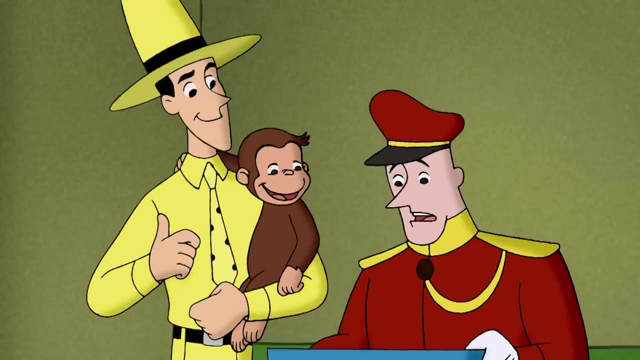 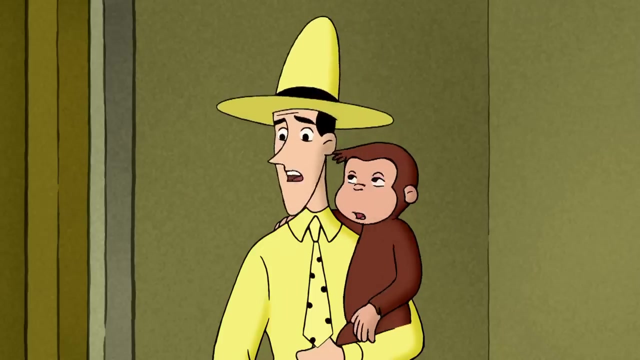 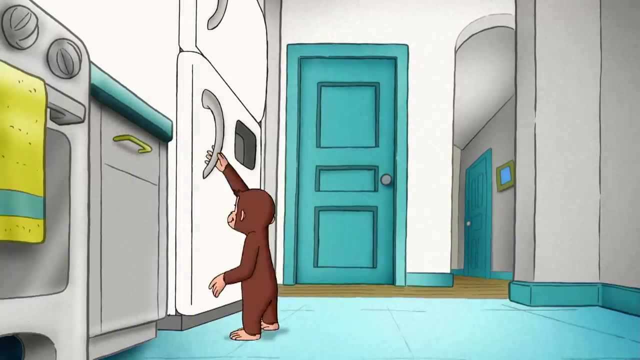 Three cans, and it's not even noon. I bet Lydia hasn't even gotten a bottle cap. Three cans, All right. Oh, maybe it's not going so well If their doorman needed recycling. George was ready to get to work. 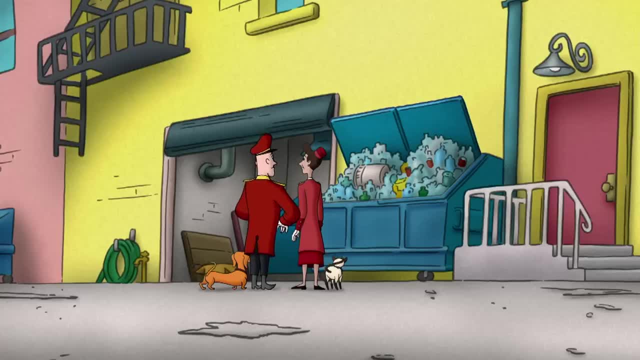 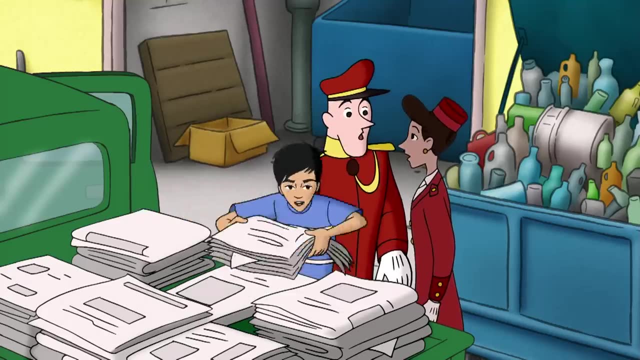 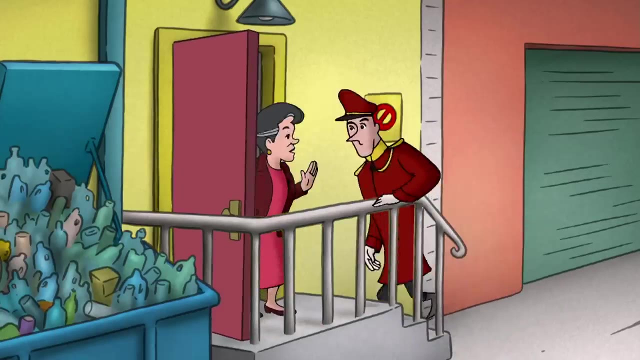 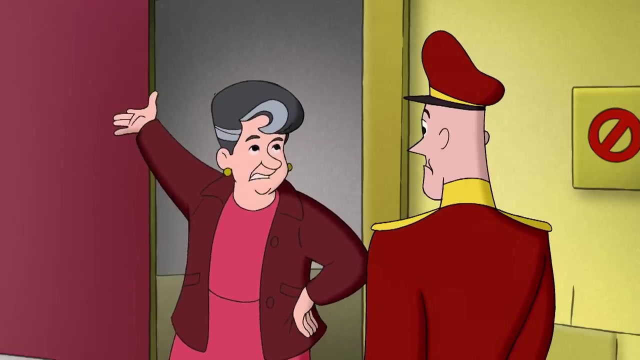 Have I? I mean, I have Nobody got their newspapers this morning. Weird, I say nothing. There you are. We have a food thief in the building. I got a grocery delivery and someone took half of it. What Someone took my paint pails. How can I mix paint with no pails? 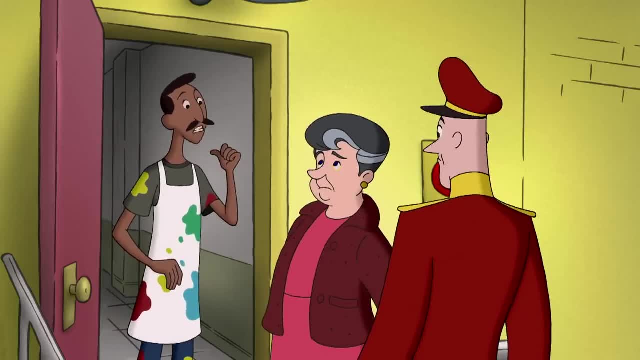 Where are the WikiPizza coupons? They're always on the front table. Huh, Oh, The company has more than one client. You've got to be kidding me. Here's a good one. Oh, Watch who's better at the box. 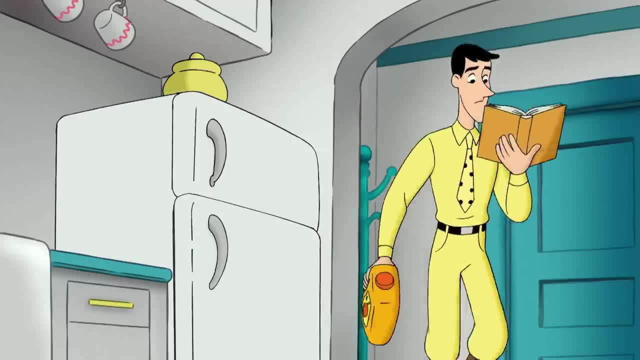 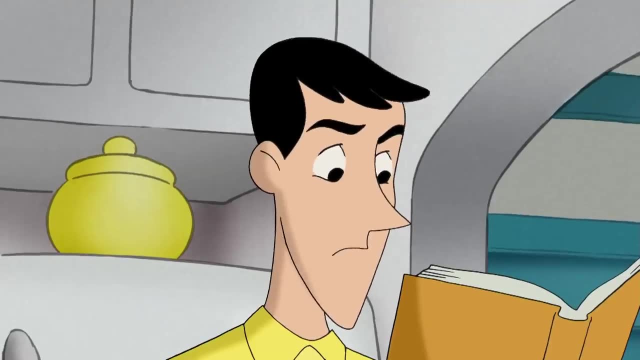 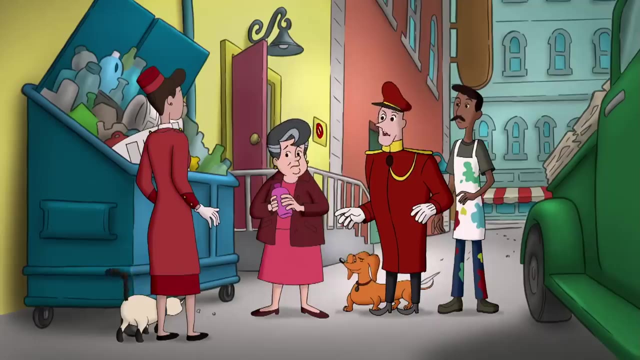 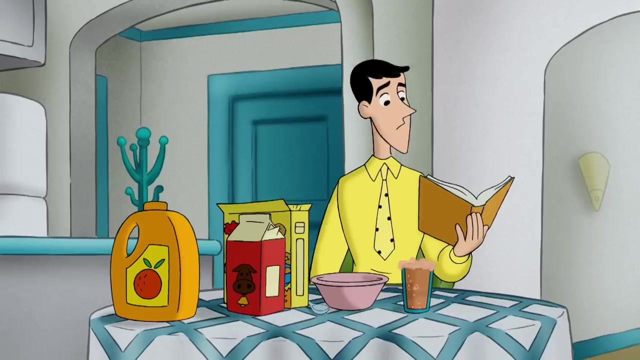 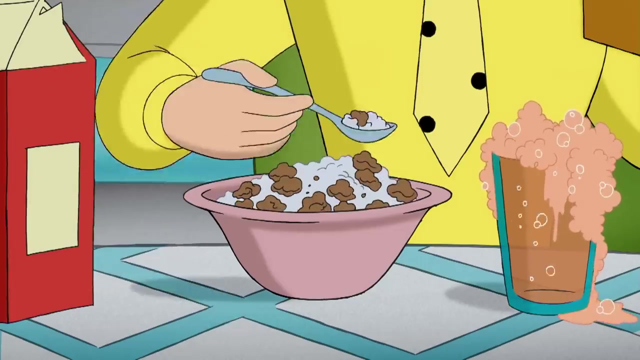 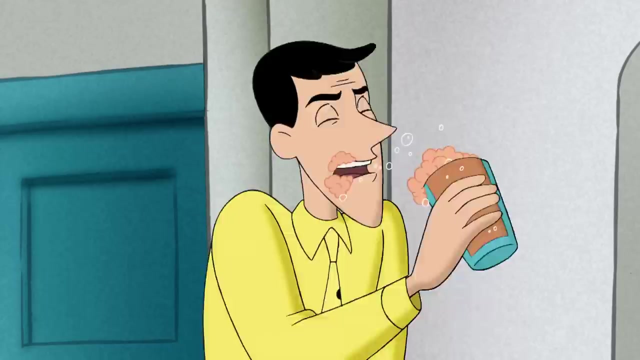 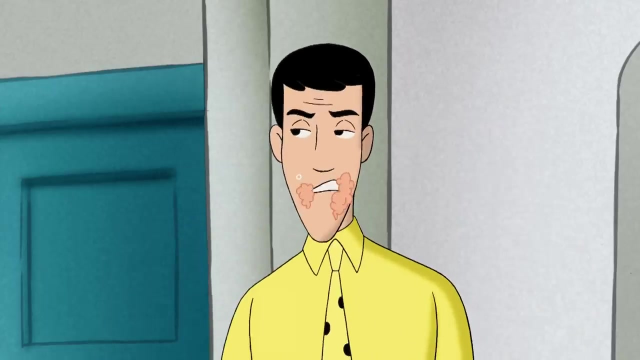 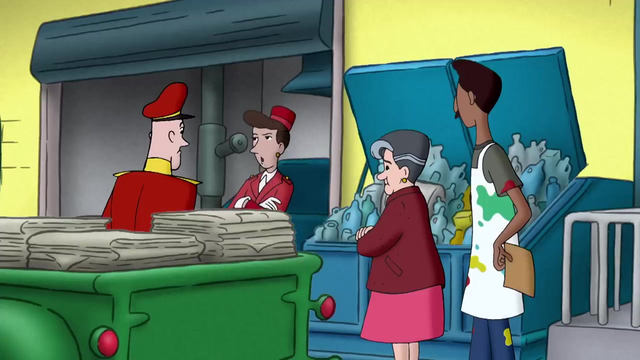 I'm Harold. See you later. See that I'm God. I need to know more about my kids. I know my kids. I can't wait. Let's go, Let's go. I don't understand what pizza coupons. Oh boy George, those things are unused. did you take them just to win the?